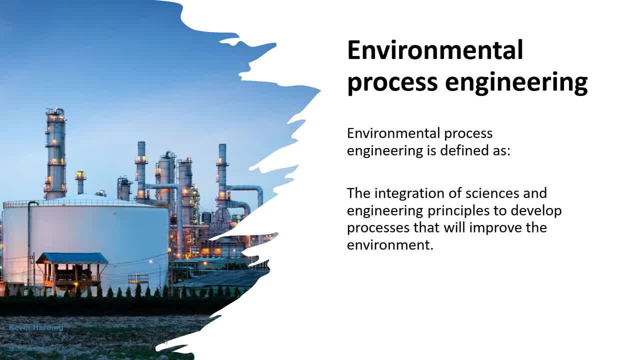 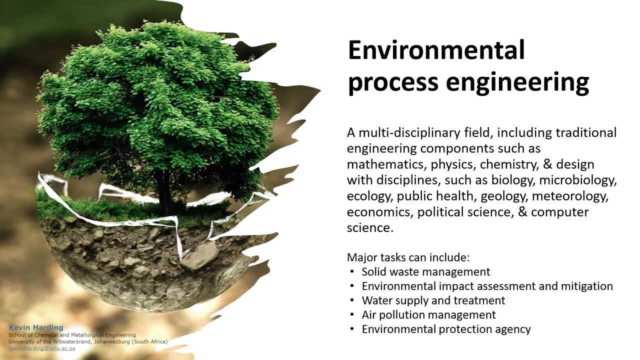 we can define environmental process engineering as the integration of the sciences and engineering to develop systems that will improve our environment. In reality, environmental process engineering is a multidisciplinary field which includes typical engineering as well as other scientific fields to solve such diverse problems. 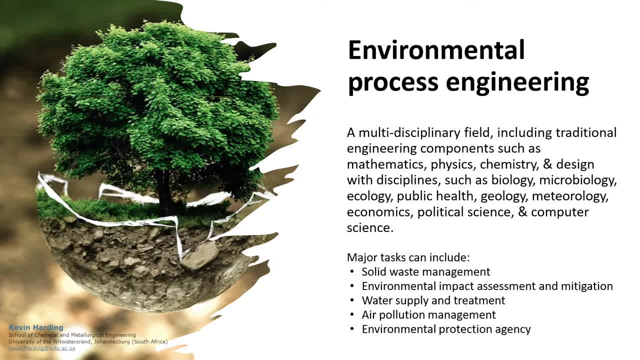 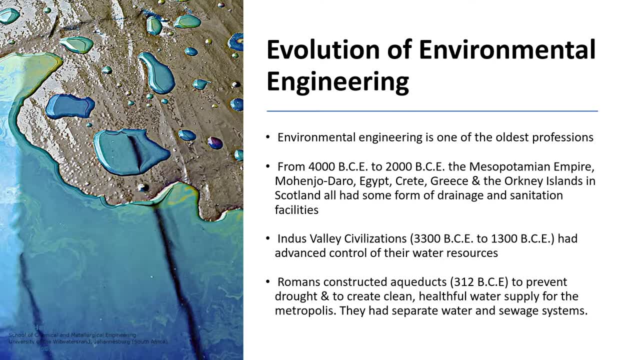 Environmental engineering is not a new field. The Mesopotamians, Egyptians, Greeks and others all had some form of drainage and sanitation facilities. The Indus Valley civilizations also had advanced control of their water resources, as did the Romans, who constructed aqueducts. 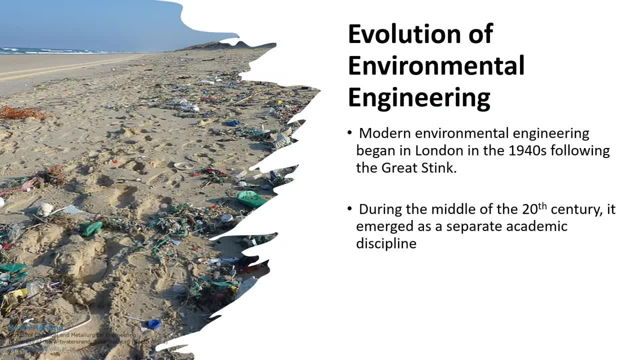 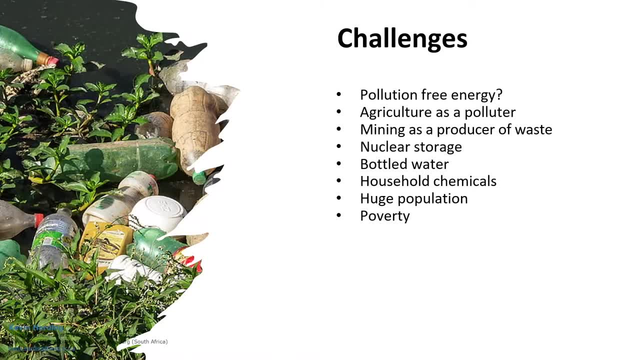 In more recent times. environmental engineering came to the fore during the Great Stink of London. During this time, it also emerged as an academic discipline of its own. Environmental engineering comes with its own challenges. Can we get pollution-free energy? Agriculture is important to all of us, yet it can contribute as a large polluter. 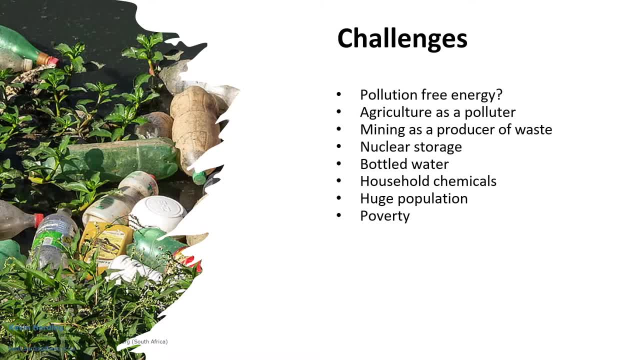 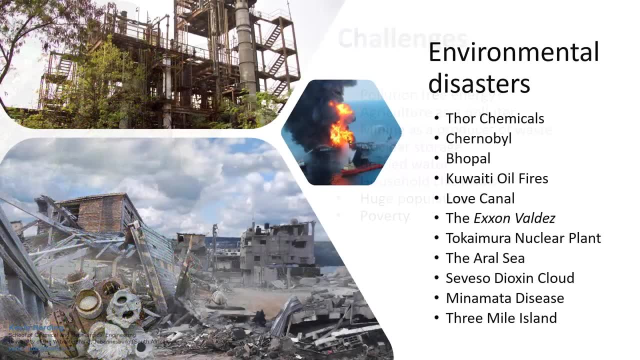 Mining is important to many economies, yet can produce large amounts of waste. Bottled water has become popular, yet empty bottles can lead to great sources of plastic pollution. There are also various examples of industrial facilities or sites that have had major incidents, which have led to avoidable disasters as well as the loss of lives. 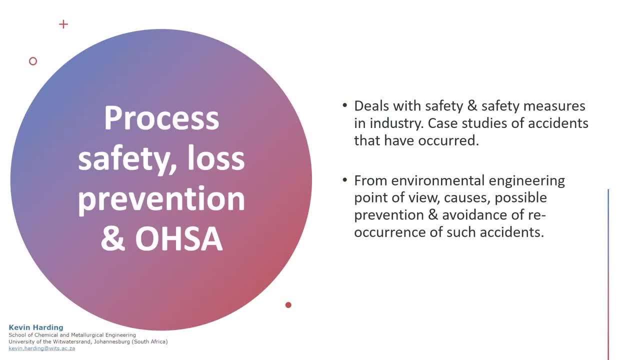 As such, we are going to talk about process safety, loss prevention and occupational health and safety as part of environmental engineering. Here we deal with the safety measures to avoid instances like these. In this course, we will look at snapshots of different aspects of environmental engineering. 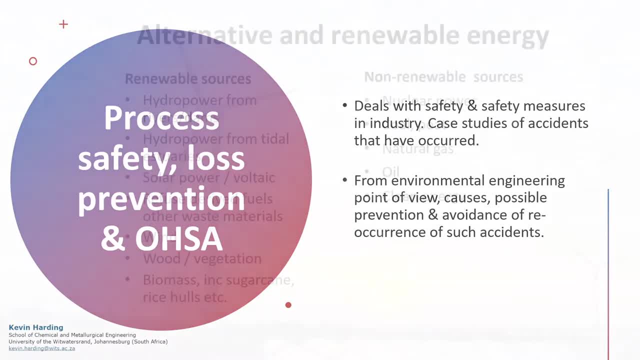 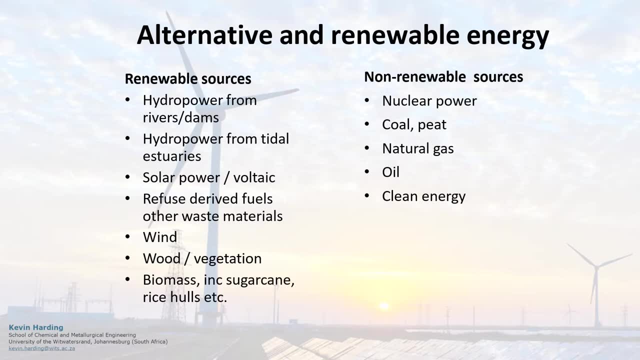 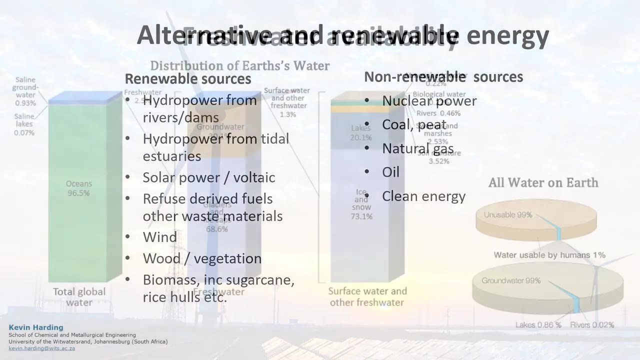 as well as ways to reduce impacts on the environment and loss of life. One of these aspects of environmental engineering will be alternative and renewable sources of energy. These include solar, wind and biomass. versus non-renewable sources such as coal, natural gas or oil, Fresh water is a vital aspect of environmental engineering. 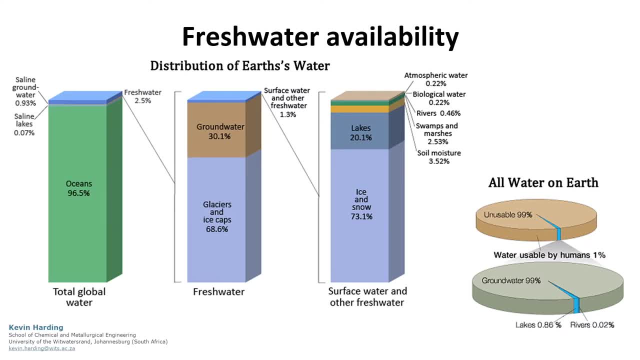 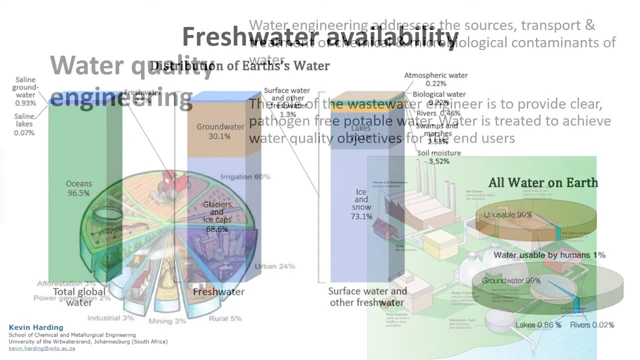 where we see that only 1% of the earth's water is available for human consumption. This makes it important to make sure that we take care of our natural resources without wasting. To make sure that we make the most of water, we are going to look at engineering measures. 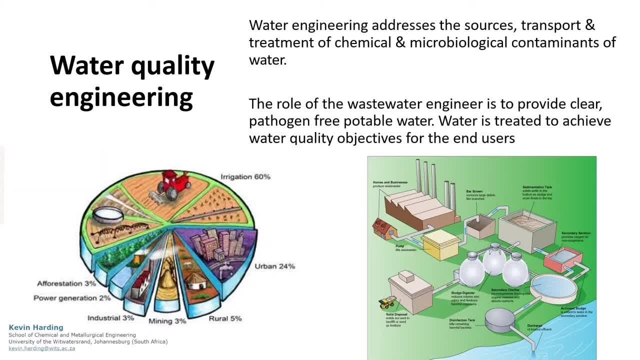 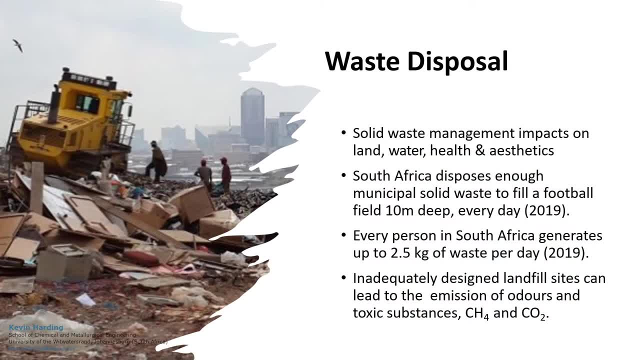 to treat water to remove chemical and microbiological contaminants. Wastewater engineers are going to be key to provide clear, pathogen-free and potable water. Environmental engineers are also responsible for proper solid waste management. In South Africa we dispose of enough municipal solid waste to fill a football field 10 meters deep.